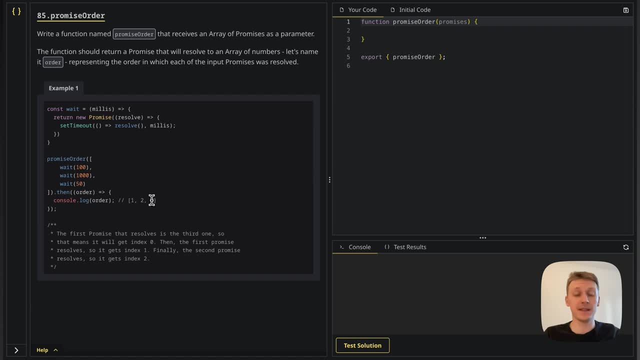 And the expected output should be this one: 1,, 2, 0.. And let's look at it and understand why. So the first promise that finishes is the third one, this one right here. That means we put here index 0, it's the first one finishing. Then the second one is going to be this one weight of 100. 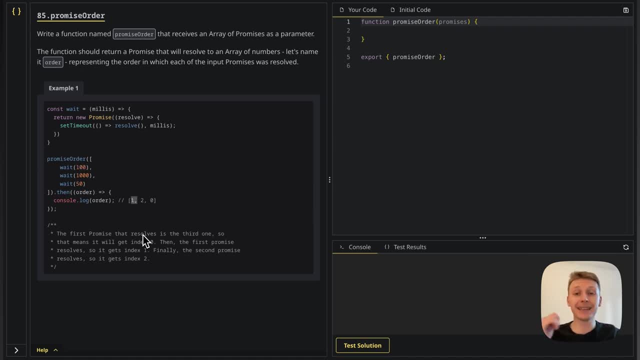 So we put here index 1.. Lastly, we get the middle promise where we're going to put index 2.. And all of those explanations are below, so you can see them in the comments here, Now that we've read the description. 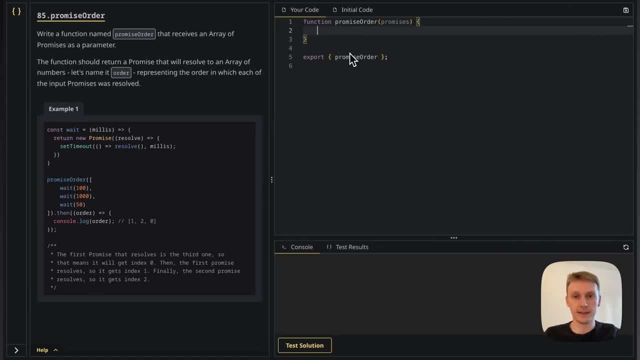 let's go into the right side, into the code area, and start solving it, And the first thing I want to do is create a new promise here that I'm going to resolve. So I'm going to say return, that I'm going to return, not resolve. sorry, New promise And then I'm going to return it here. 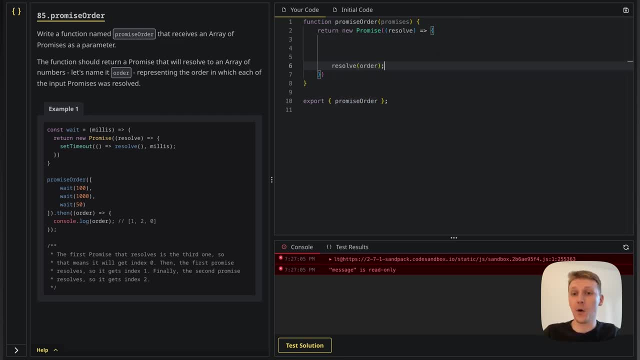 And this one is going to resolve with an array. We're going to call order, So let's just create it. const order is initially, let's say it's empty. Okay, now the challenge is: what do we write inside? Because I need to wait for all promises to finish. 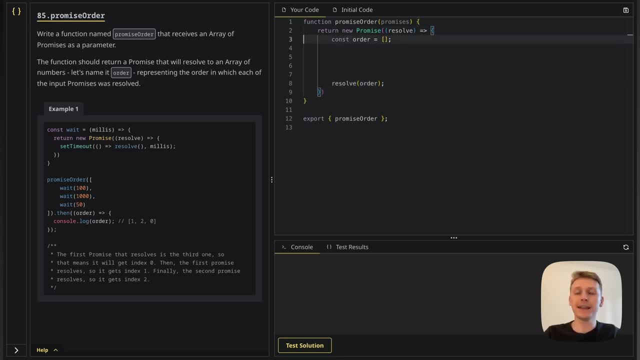 before I resolve this right. So I'm going to create a new variable here. So I'm going to say: let promises finished is equal to 0. And I'm going to do a 4., 4, or actually I don't even need to do. 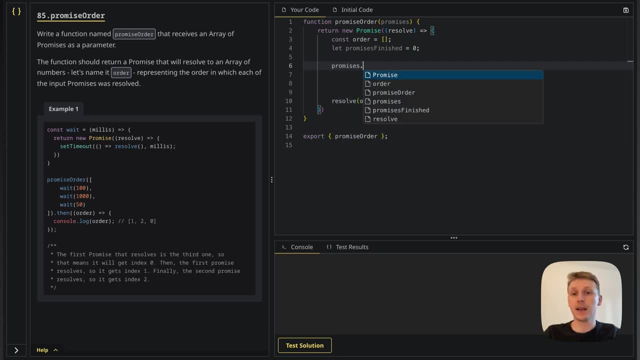 a 4. I can do a for each. So I'm going to do: And here I get a promise, right, So I get a promise. and then I'm going to say something like this: I can do an async, await, async here and I'm going to say: await promise, So I wait for. 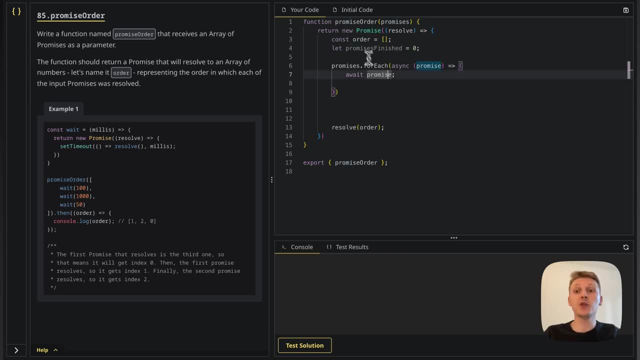 this promise to finish. Now that this one finished, I need to put the correct index to its position. So I'm going to get its position from here. so index- and now I'm going to do order of index- is going to be promised. promises finished, right? so if this one is the first one that finishes,